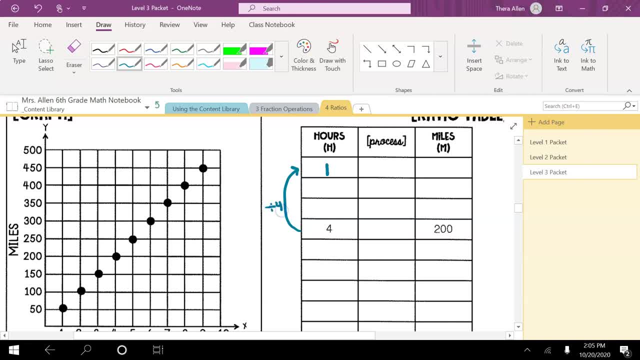 Well, I know that I divided by four, And if I do that there, I have to do it here as well. Divide by four And 200 divided by four is 50. So it actually is going to be 50.. Now let's look at the process. 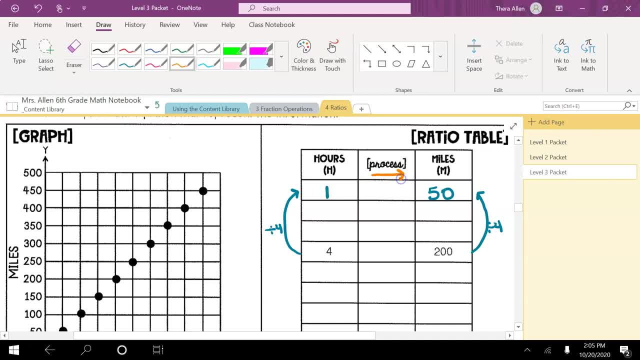 Remember the process. The process is telling me what's happening across. Also, remember that this is our x-axis, This is our x-axis And this is our y. Okay, Let's look at the process To go from one to 50, I am multiplying the hour, which is one times 50.. 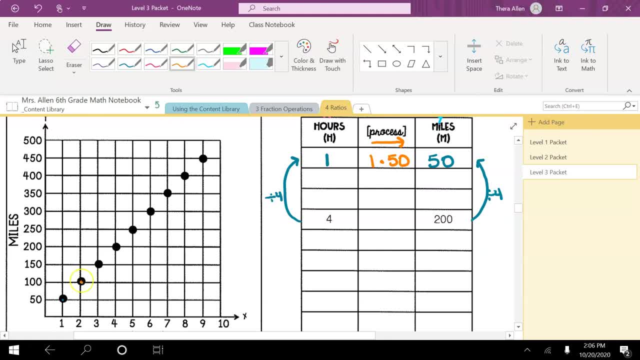 Okay, Now we're moving to our next plotted point, which is right here, Which is two. So we're going to put two, And if I keep looking, I notice that they're all the way down to nine. So three, four, five, six, seven, eight, nine. 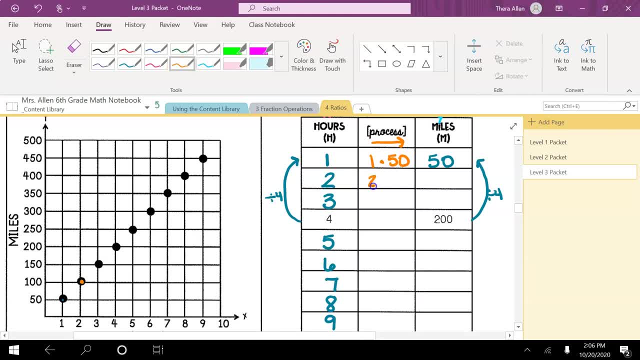 And my process every time is going to be taking the hour multiplying by 50. The hour times 50.. The hour Times 50. And continuing on until I get to nine times 50. If I keep on going, I will end up with finding my miles, which we know actually does match. 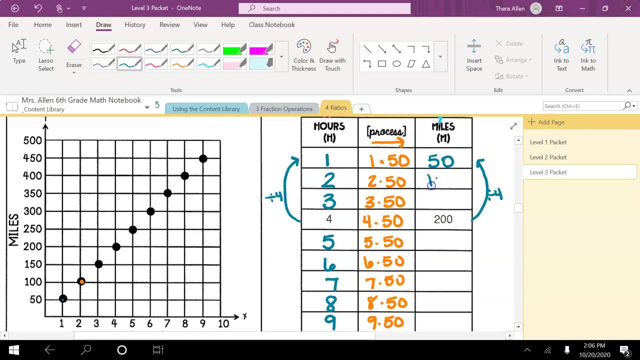 up to the graph, but it does not always. So. two times 50 is 100.. Three times 50 is 150.. We already have four times 50.. Five times 50 is 250.. Two times 50.. Six times 50 is 300.. 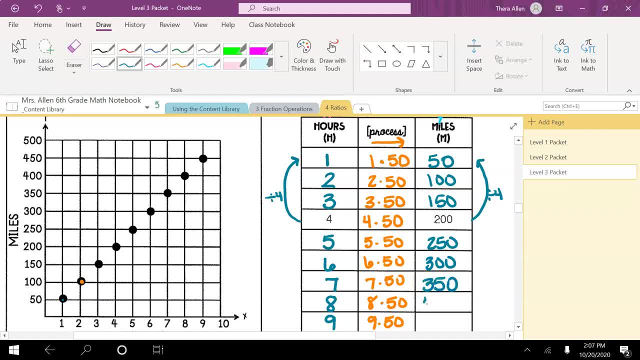 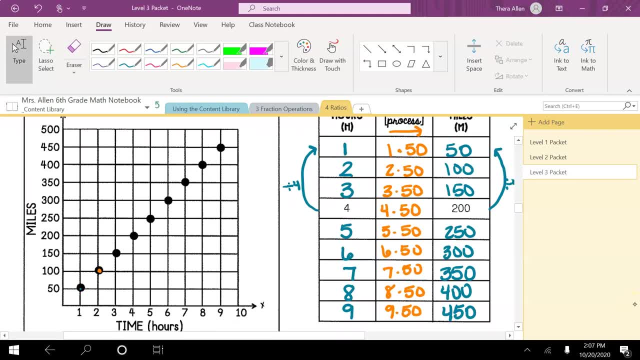 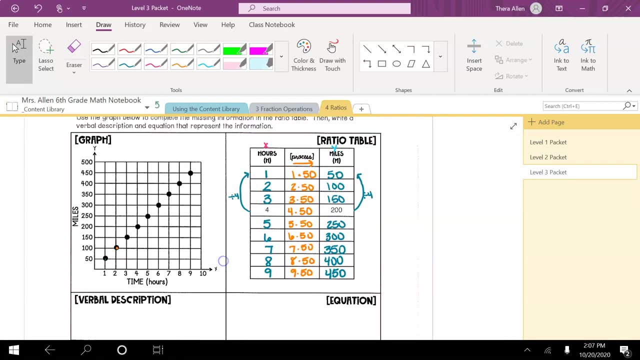 Seven times 50 is 350.. Eight times 50 is 400.. And nine times 50 is 450.. So now let's move down and let's do a verbal description. Well, to describe this graph, we see that we have time. 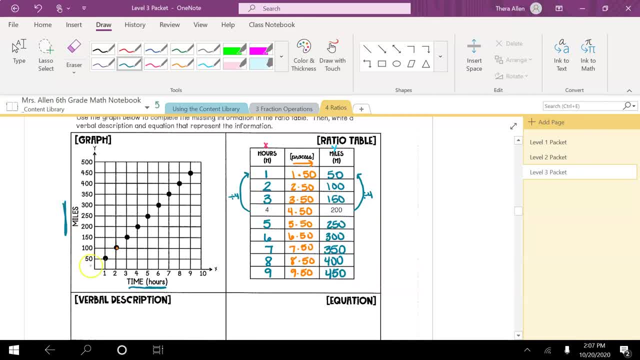 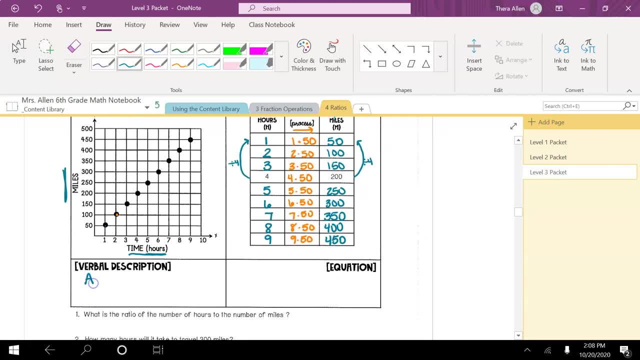 So in one hour something is traveling 50 miles, And I would just think of a car. So for I would say, a car travels 50 miles in one hour. Okay, You're going to. normally, when you are describing your ratio, you're going to use the simplified. 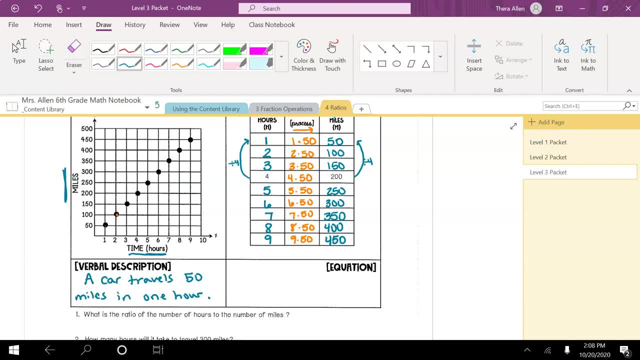 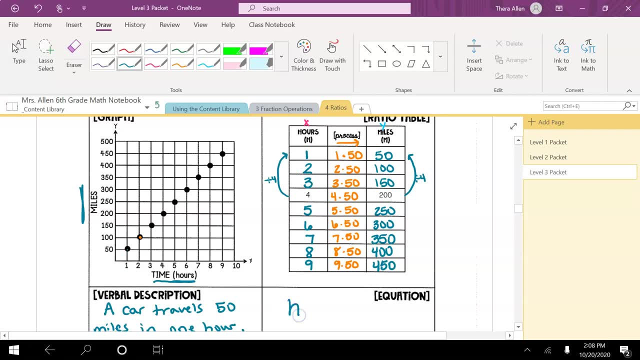 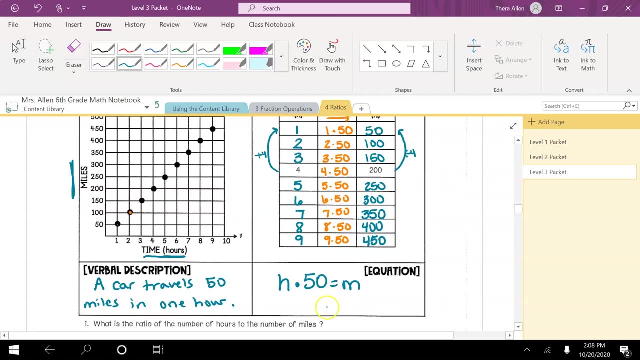 ratio. So you're going to use the simplified version of your ratio And then for an equation, remember, we have the hours. We look at the process. It is the hours times 50, which gives us the miles. And another way that we can write that is: miles equals 50H. 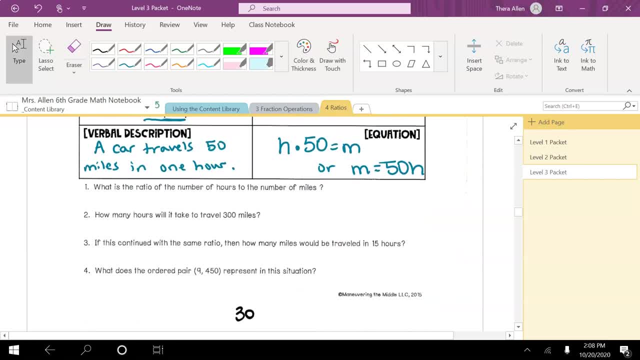 Let's move on down and answer these questions. What is the ratio of the number of hours to the number of miles? That's what asking you. the simplified ratio- The number of hours was one- to the number of miles- is 50. So how many hours will it take to travel 300 miles? 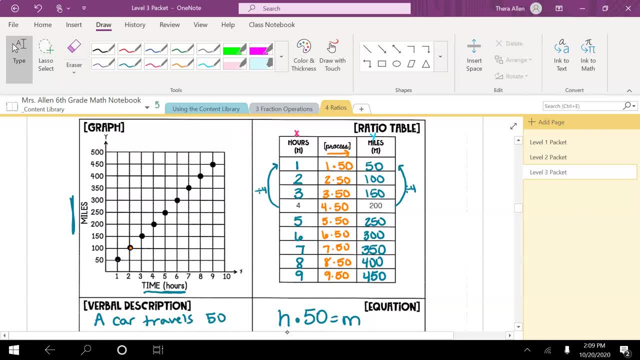 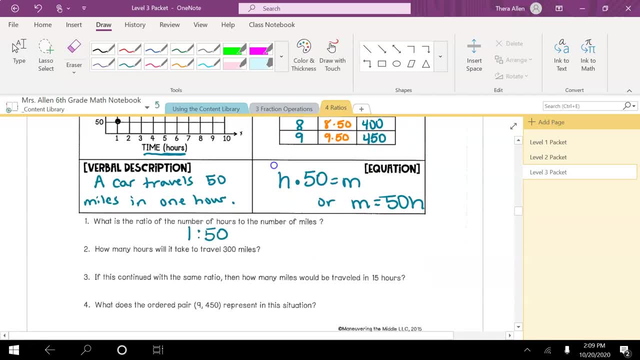 Well, we can look on our chart here on our table And I see right here 300 miles. So it would take six hours. So our answer here is six hours. If this is continued with the same ratio, then how many miles would be traveled in 15 hours? 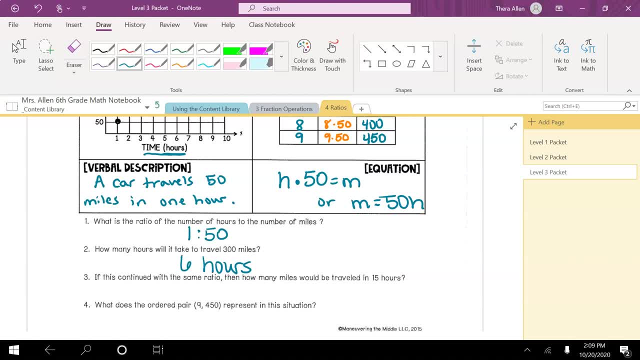 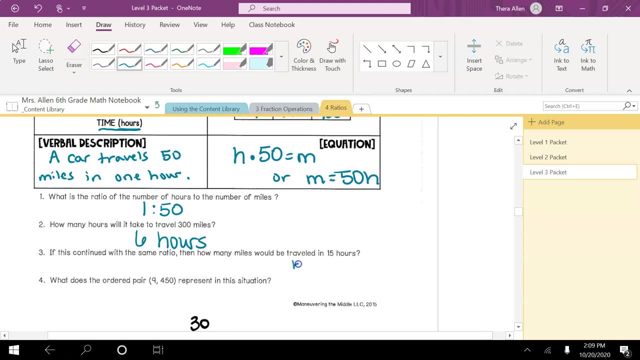 Now there's a couple of ways that you can do this. You could set up a proportion, or you could look on your table To set up a proportion. you would say, okay, I'm going to do hours over miles, So that's one hour 50 miles. 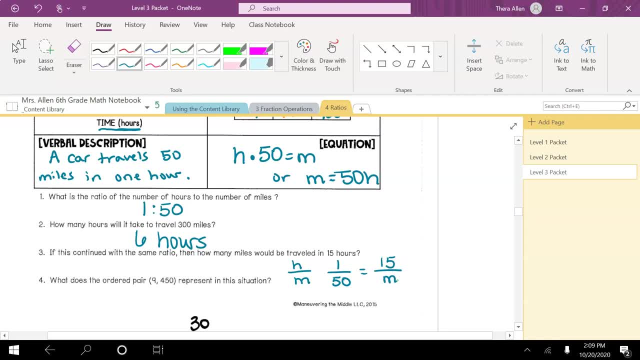 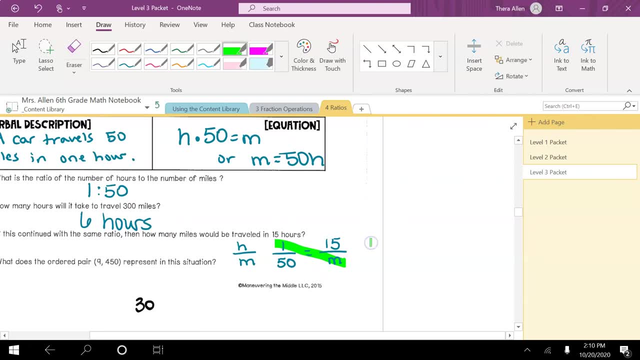 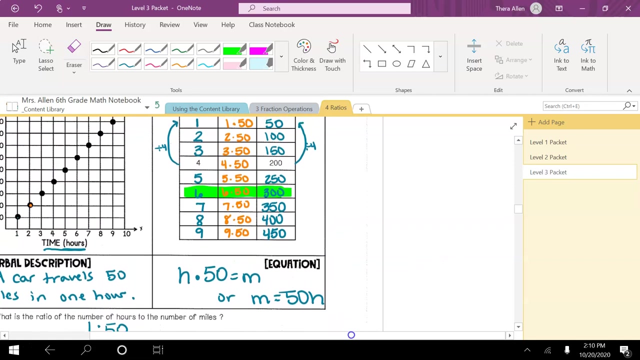 And I want to know 15 hours equals how many miles. Then I do my cross, multiplying One times M is M, And then I say 50 times 15.. Okay, and 50 times 15 is 750.. I could also look up here and I could say: okay, 15 miles. 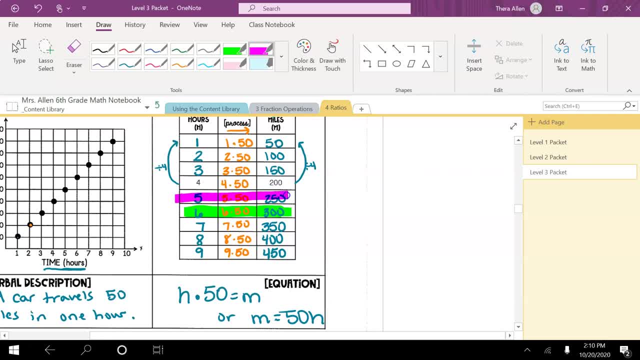 Well, I'm going to look right here at this part of my table And I'm going to say, okay, well, five can go to 15 by multiplying by three. So 250 times three gives me 750 miles. Same way, just whichever is easiest for you to think about. 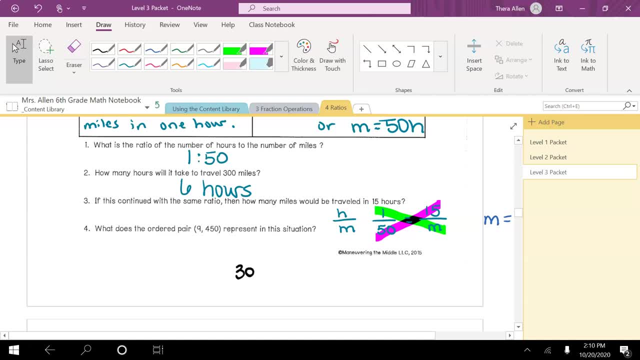 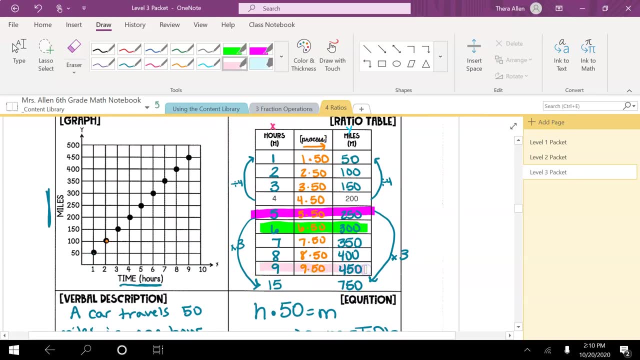 What does the ordered pair, 9, 450, represent in this situation? So let's go back and look Right. here we have 9 and 450.. This 9 represents how many hours and the 450 represents the number of miles. 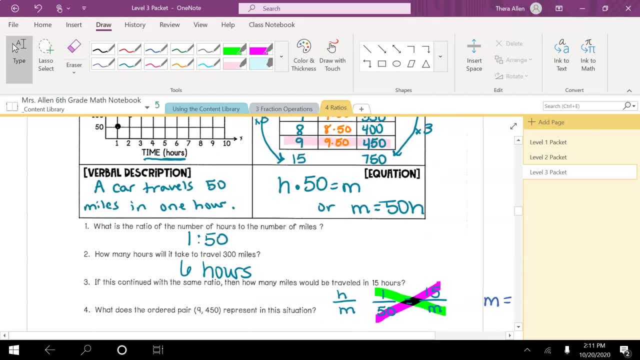 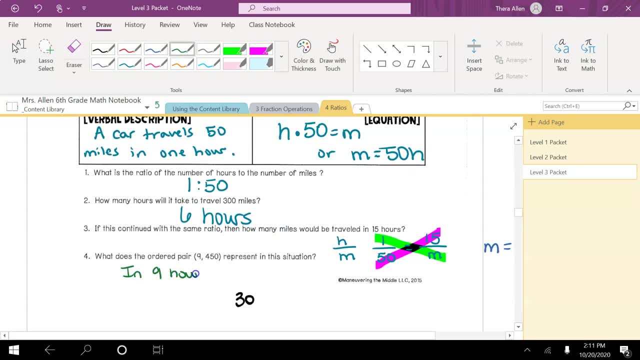 So this represents that in nine hours they traveled 450 miles. So in nine hours we'll say the car traveled 450 miles. We are learning how to put a number in the right place. We are learning how to put a number in the right place. 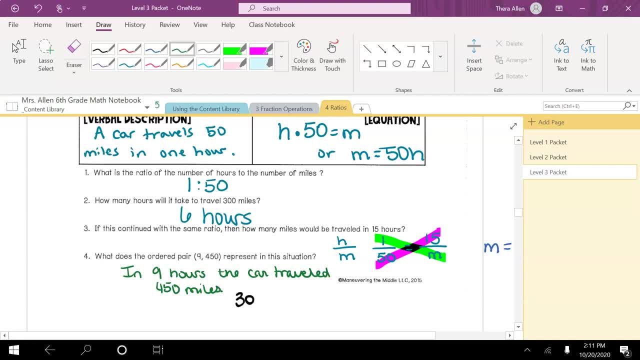 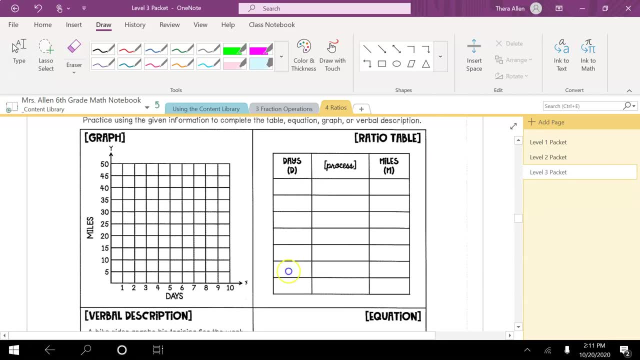 We are learning how to put a number in the right place. We are learning how to put this information into word form. All right, let's go on to the back. We're on page 31.. We are going to practice Now. this time they did not put anything on the graph. 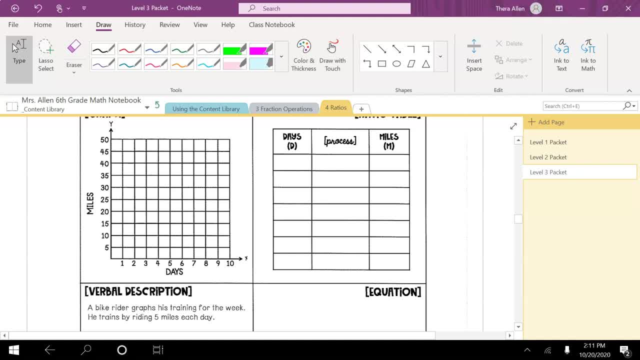 They just gave us the information down here, the verbal description. The verbal description says a bike rider graphs his training for the week. He trains by riding five miles each day. I prefer making the table first. So five miles each day. Well, so that means at one day one he trained five months. 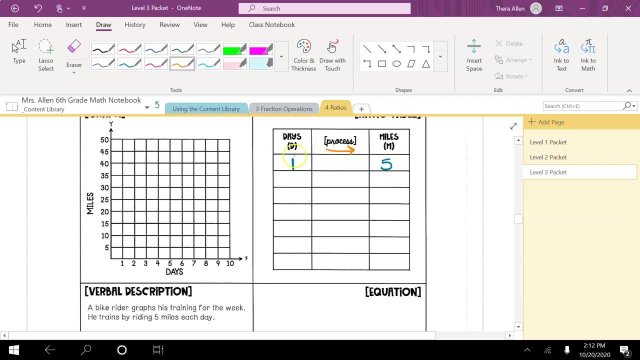 And that means my process is taking the day multiplying by five, And then we can move on to day two, three, four, five, six, seven, And then each one of these is the same process. We're taking the day multiplied by five. 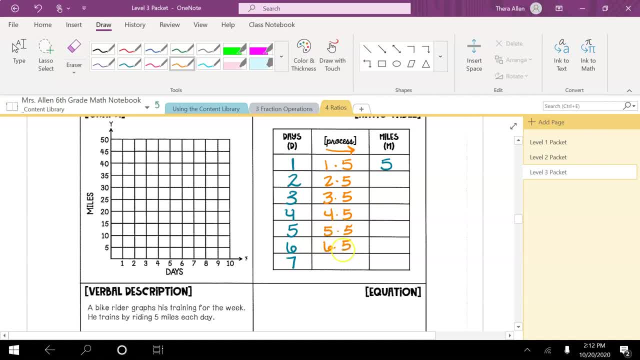 Five. so we're going to write that all out in our process area And then we are going to write the actual miles. So two times five is 10,. three times five is 15,. four times five is 20,. five times five. 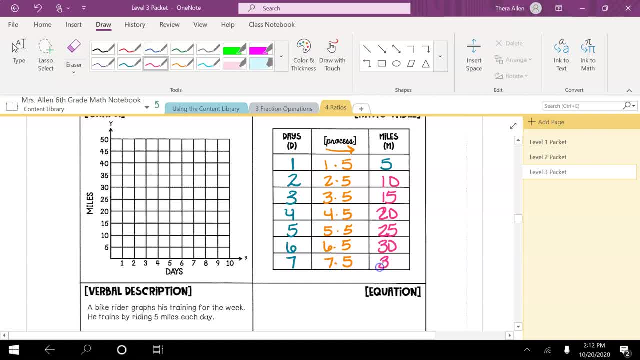 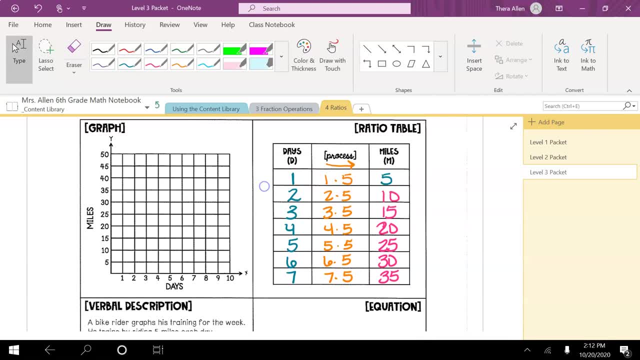 is 25,, six times five is 30, and seven times five is 35.. Now I can take this information and plot it, But before I do, I need to remind myself that this is my x-axis And this is my y-axis. 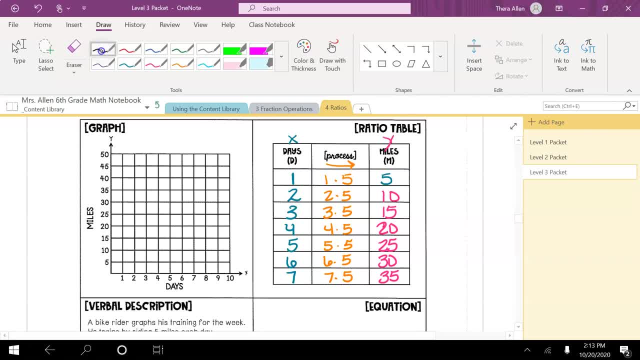 So my first ordered pair is one five. So I'm going to go to one five and put my dot. Then I'm going to say two to 10, my dot three to 15,, four to 20,, five to six. 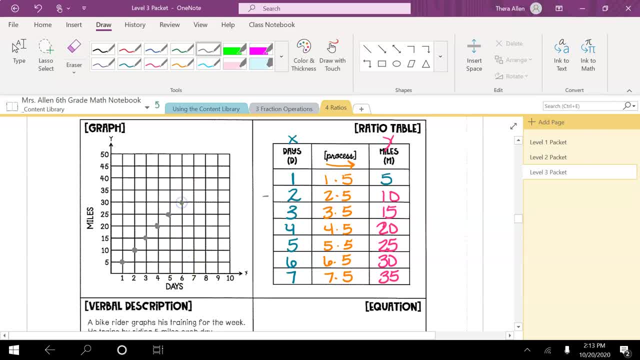 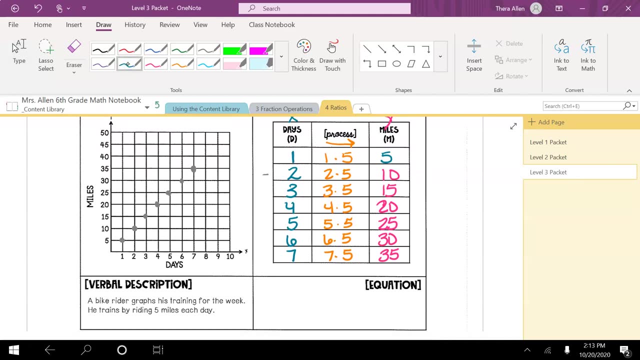 I'm sorry, five to 25,, six to 30.. Seven to 35. And I could actually follow the pattern and keep on going, But I'm going to stop right there. Now I want to write an equation, So I'm going to say: remember, here in my process it shows me. 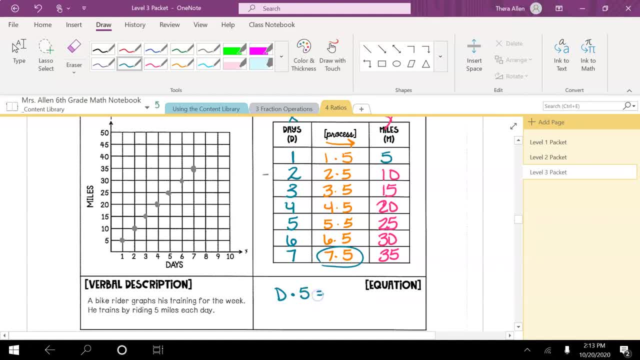 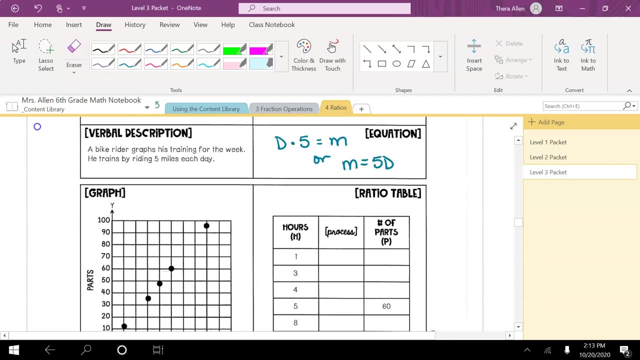 I take the number of days times five and that gives me the number of miles. Or I could write it as: the number of miles equals five times d, And that's the way I can write it. Okay, we are going to quickly look at this one. 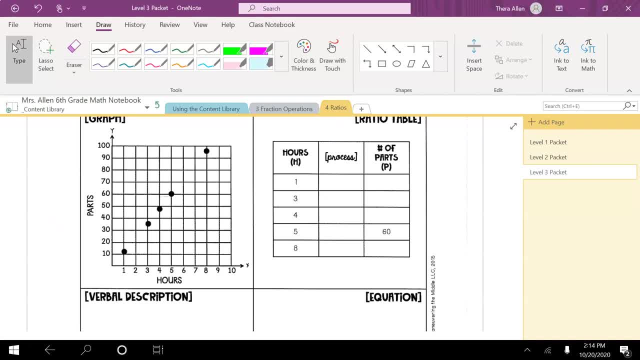 I'm not going to worry about the verbal description or the equation right now, But I want you to look if you notice they've skipped a little bit, So we don't have this one, this one or this one, but that's okay. 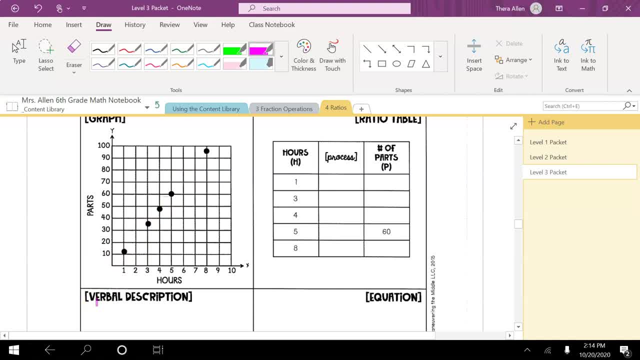 We don't need them. So let's look. remember that does not quite look like it is at the 10.. So let's see, Let's go over here And look: five divided by what gives me one? Well, divided by five. 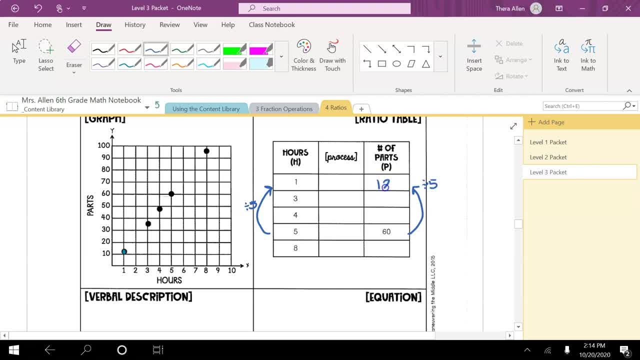 So 60 divided by five gives me 12.. Now I can figure out my process. My process is going to be the hours times 12.. So this- I look at my hours- which is three times 12,, four times 12,, five times 12,.